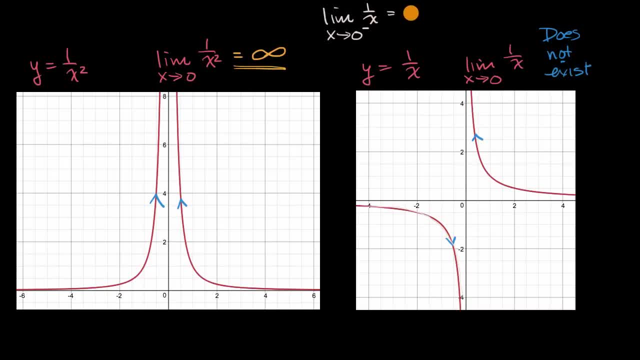 well, look, it looks like we're going unbounded in the negative direction. So you would say this is equal to negative infinity. And, of course, if you said the limit as x approaches zero from the right of one over x, well, here you're, unbounded in the positive direction. 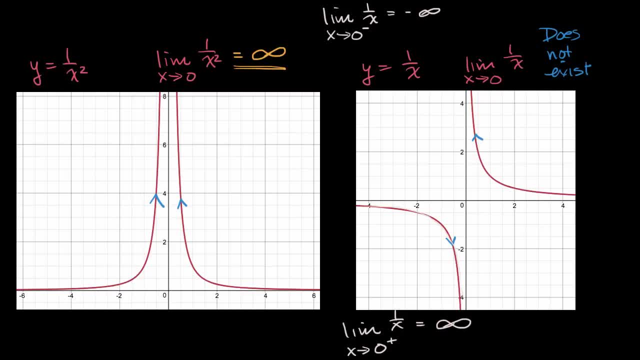 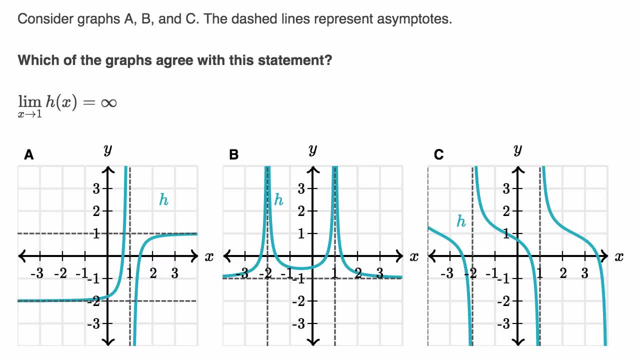 so that's going to be equal to positive infinity. Let's do an example problem from Khan Academy based on this idea and this notation. So here it says: consider: in graphs a, b and c, the dashed lines represent asymptotes. 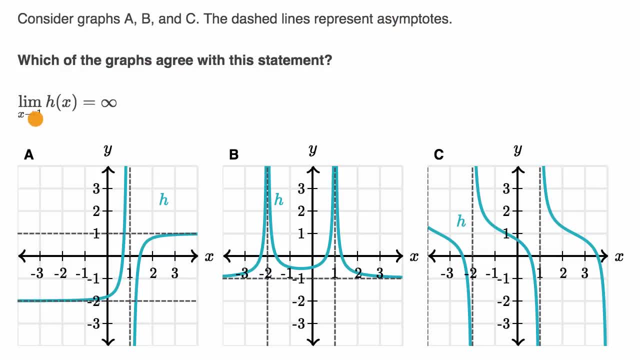 Which of the graphs agree with this statement that the limit as x approaches one of h of x is equal to infinity? Pause this video and see if you can figure it out. All right, let's go through each of these. So we want to think about what happens at x equals one. 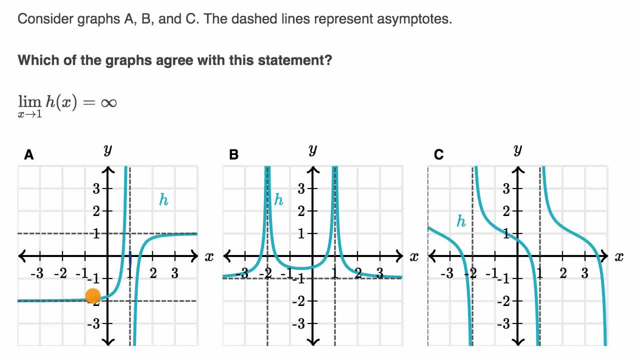 So that's right over here on graph a. So as we approach, x equals one. so let me write this. So the limit, let me do this for the different graphs. So for graph a, the limit, the limit as x approaches one from the left. 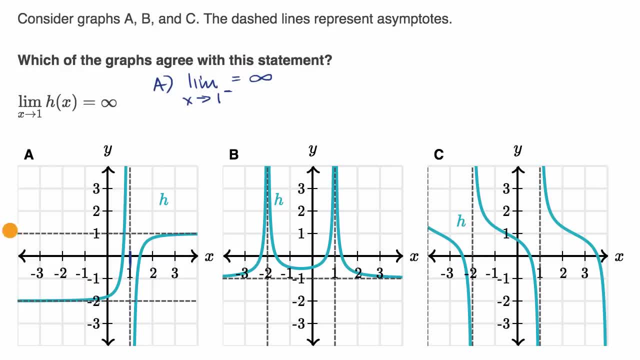 that looks like it's unbounded in the positive direction. That equals infinity. And the limit as x approaches one from the right? well, that looks like it's going to negative infinity. That equals negative infinity. And since these are going in two different directions, 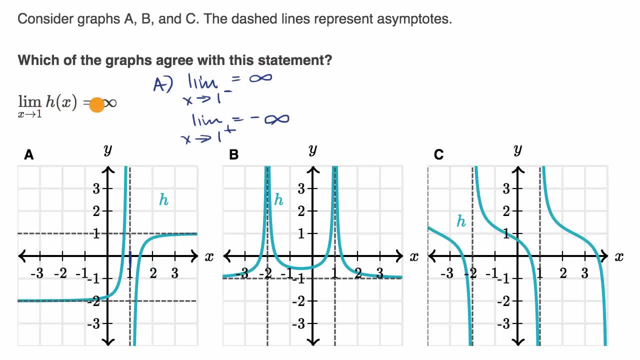 you wouldn't be able to say that the limit as x approaches one from both directions is equal to infinity, So I would rule this one out. Now let's look at choice b. What's the limit as x approaches one from the left? And of course these are of h, of x. 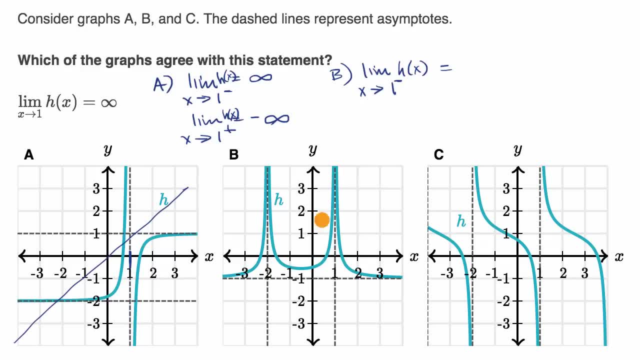 Gotta write that down. So of h of x right over here. Well, as we approach from the left, we are going to looks like we're going to positive infinity And it looks like the limit of h of x as we approach one from the right is also going to. 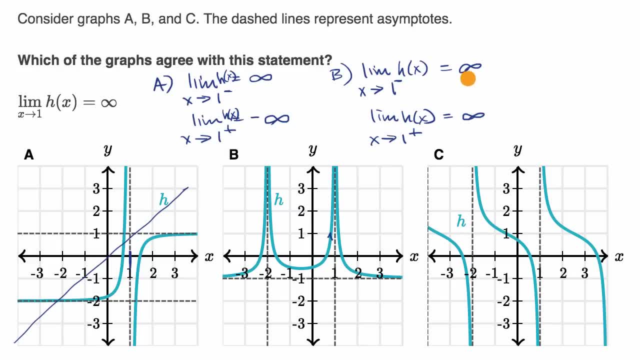 positive infinity. And so, since we're approaching, you could say, the same direction of infinity, you could say this for b. So b meets the constraints, But let's just check c to make sure. Well, you can see very clearly: x equals one.